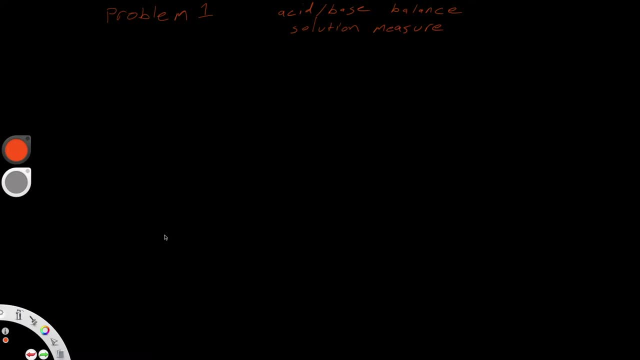 Hello and welcome back to another episode from iWater Studio. Today we're going to be talking about the Fundamentals of Engineering exam, specifically for environmental engineers. Now, you probably already know about this exam if you're watching this video. It's basically a four-hour. 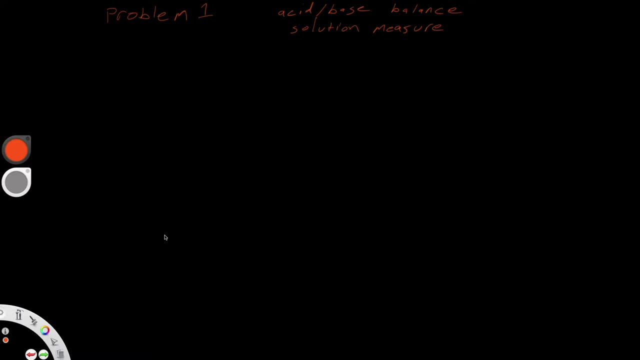 exam in the morning over general engineering principles, like your engineering sciences, and then it's followed by a four-hour exam in the afternoon focused on your specific field of study, And so we're going to focus on environmental engineering for that second half. Super challenging test for. 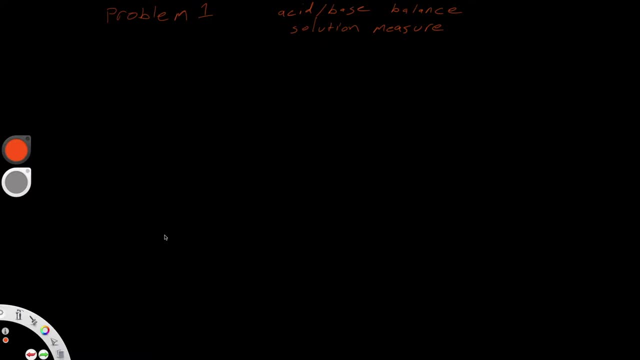 for new engineers, for recently graduated undergrads or about to graduate undergrads. I'm going to try to you know, see what the interest, what kind of interest there is in this exam. I'm going to focus on this and we're going to run through three problems real quick and talk a. 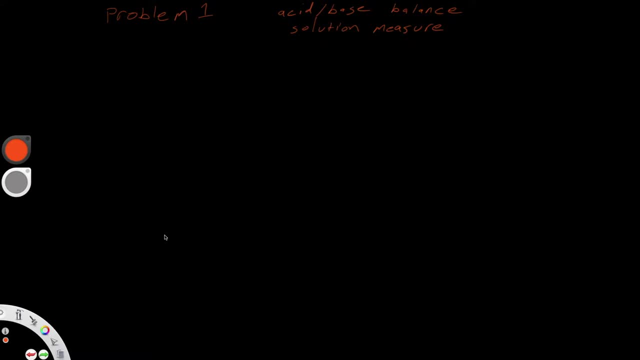 little bit about how they might apply to the exam. So our first problem. actually, I wish I would have wrote the problem out already. Oh, there, it is Okay, sorry. So the first problem- that's pretty common- is going to be some kind of measuring out of a solution: How to dilute a solution, prepare a solution or 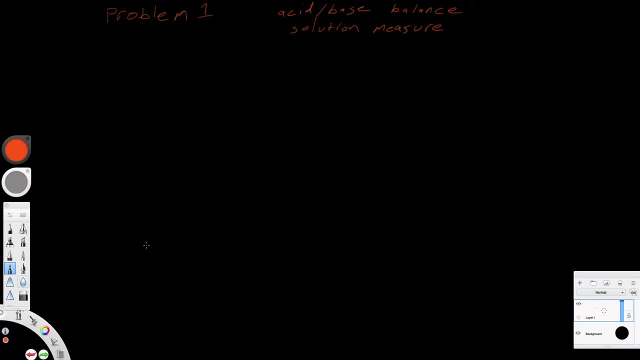 balance a solution, something like that. So the one we're going to look at and actually solve here is going to be neutralizing an acid and base. So, for example, if you have a four molar solution of a very obviously very common acid, hydrochloric acid- and you want to add that to neutralize, 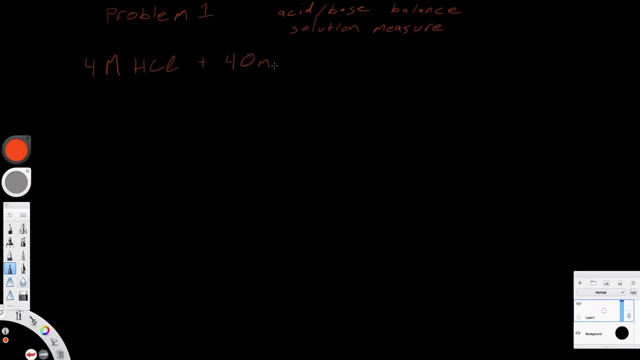 higher saturate inside that acid. the acid and base helps to provide this solution, which is Cer Brisbane, and this might be ready to be applied. So we're going to be mixing in 40 milliliters of, you know, two kind of Casa or four, 40 milliliters of a six. 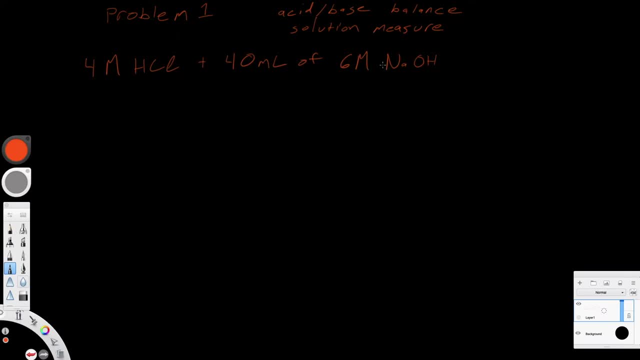 molar solution of sodium hydroxide. Obviously, molar is moles per liter, and so this is relatively simple, because in this case we have monovalent acid. We only have one hydrogen: one hydrogen and one hydroxide sourced into the Lulu on brilliant acid bases. 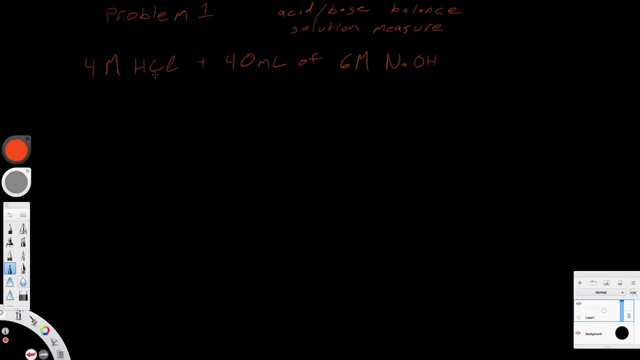 per mole. So when this, this is going to fully dissociate. both of them are going to fully dissociate because they're strong acid, strong base, And you're going to get- in this case, you're going to get- four moles of hydrogen per liter, You're going to get six moles of 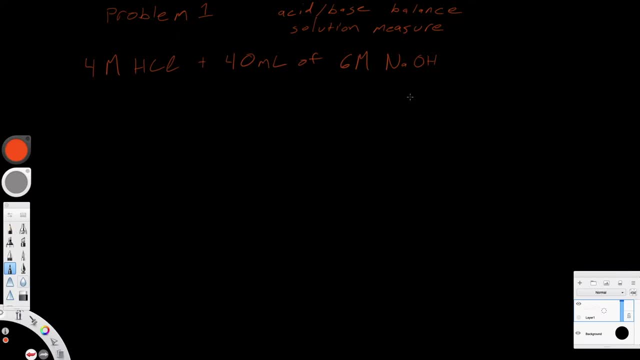 hydroxide per liter, right. So it's pretty straightforward. In this case, you just need to do a, basically a weighted average between the two. So what we do- and we do this all the time in our labs for preparing standards, and maybe I'll talk a little bit more about it afterwards- 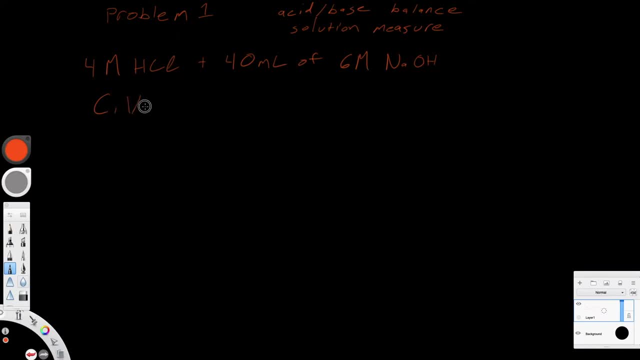 but it's basically C1,. oops, B1 is equal to C2V2.. So in this case we know C1, actually I'm just going to go ahead and say four times V- is going to be equal to. 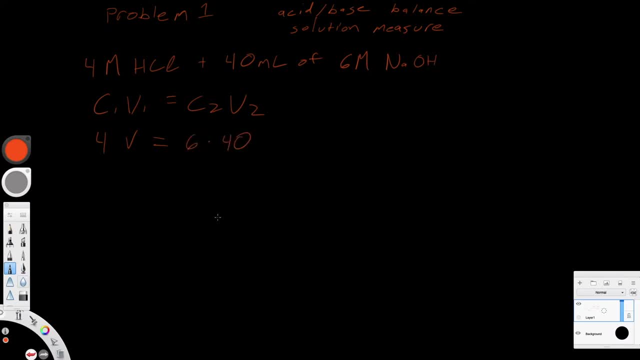 to six times 40, right, And so if you solve for V, you just have 60 milliliters, And that's I mean. you can take a look at the units and everything you know. obviously they're going to be equal, But what we can talk about is some of the things that they might try. 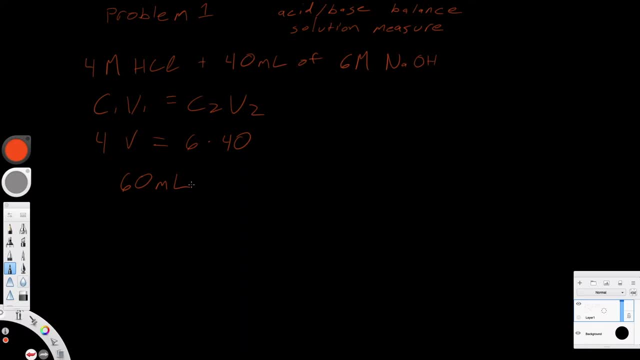 to do to throw you. You know this works because, like I said, they're monovalent. If you had something like sulfuric acid, you know this works because, like I said, they're monovalent. So, if you had something like sulfuric acid, you know this works because, like I said, 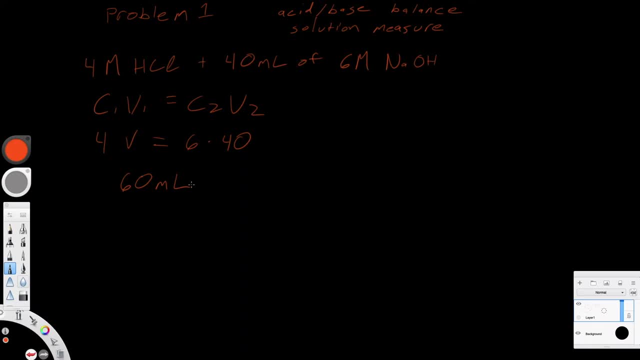 Acetic acid. this isn't going to work, at least not as easily, because you're going to have hydrogens coming off at different pH values, right, Your second hydrogen is going to come off at a different pH value and you're going. 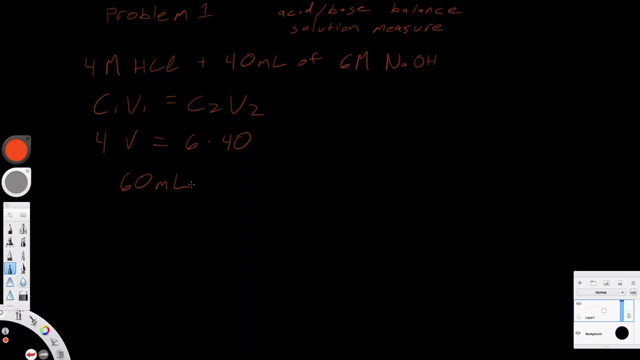 to have different equilibriums, because it's not exactly the same as being a strong acid, at least not a monovalent strong acid. Another thing they might try to do is make you use some of the molecular weights. So if they were to say something like you want to make 10 milligrams per liter silver. 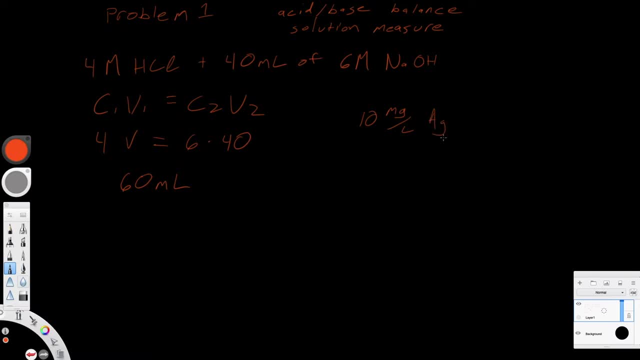 solution using, So using- Okay, 10 milligrams per liter of silver nitrate, And so obviously you can't just weigh out 10 milligrams into a liter and get 10 milligrams of silver right, Because you need to look at the molecular weight between the two to see how much. 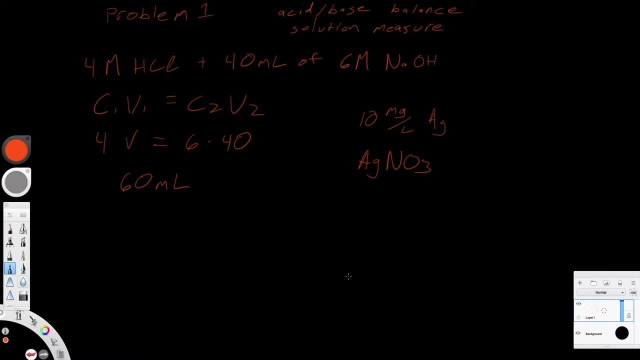 You're going to need more silver nitrate to get 10 milligrams per liter of silver, So hopefully that makes sense. Okay, And so let's. Can I just clear all of this? Although I can, It's been a while. 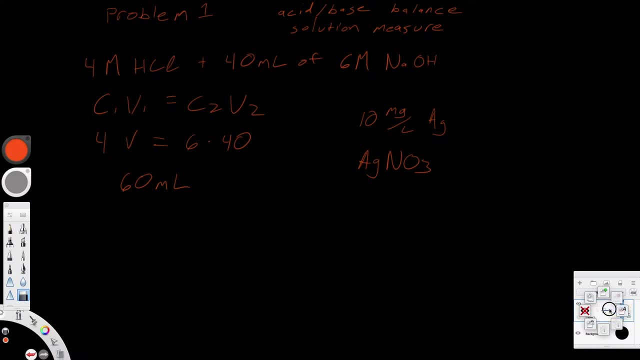 Let's just do it here, All right. All right. so another one that you're going to see, almost, I mean, I don't want to say certainly, because it's a little bit more than one liter per liter, As much as it is. 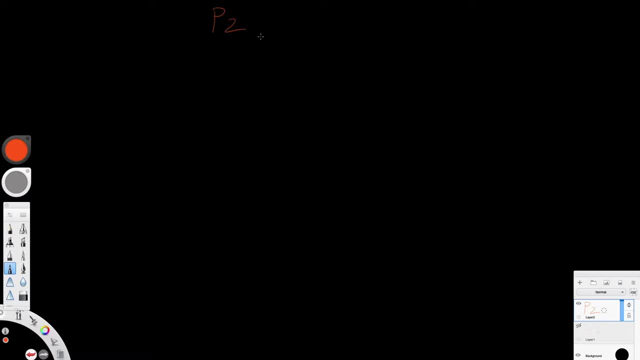 So the only thing to remember is that if it's not one liter per liter silver, then if you put 2 liters into that bottle, then probably This is so expensive. anything can be on there, but you're probably going to see some kind of 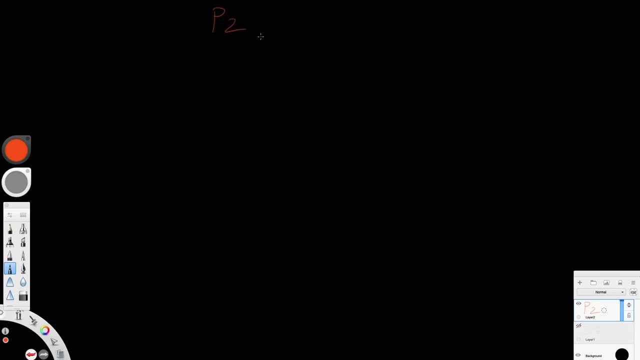 problem about decay and we actually have a video that talks about. that talks about decay in a stream. actually it's going to be pretty similar, but we're going to work it backwards. so in this case, we want to see benzene decay and we're going to have the. we're basically going to give you all the information. 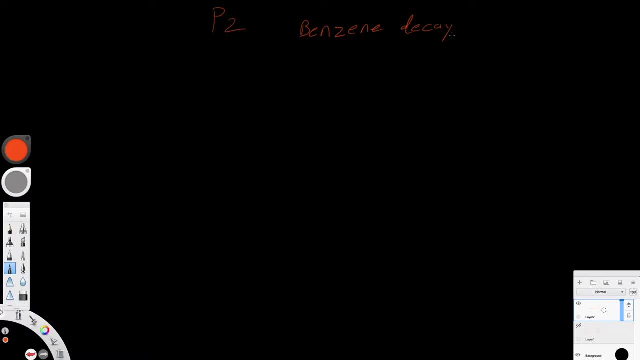 except we want to find out what is the original concentration. we're going to back calculate to the original concentration, so we know that in this case our decay rate is going to be 0.20 per day. our time that we are taking our measurement is 12 days. so in other words, benzene has been in the environment for 12 days and 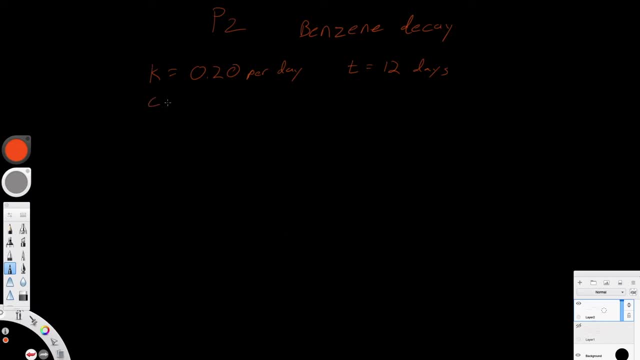 then we measured it and our concentration at 12 days, or CT, is going to be- in this case we'll just say it's 8 milligrams per liter- and so we want to find CO, our original concentration. so the basic equation for first-order decay- so benzene in this case- is going to be: 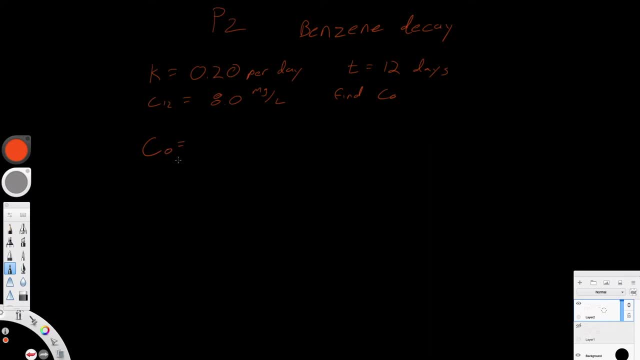 first-order decay, and it's. they're almost certainly going to tell you that, or they might. the whole question might be: just what is the decay order, decay rate? so in this case, for a first-order decay, we're going to have the original concentration and it's going to be equal to concentration at some time in the 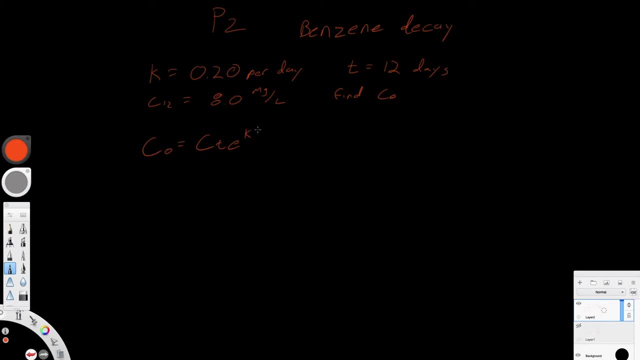 second order. so we're going to have E to the decay rate times time and if you want to know how we get this, I believe we talked about that in our decay rate video that we have. so if you, I mean, really it's just a plug-and-chug at this. 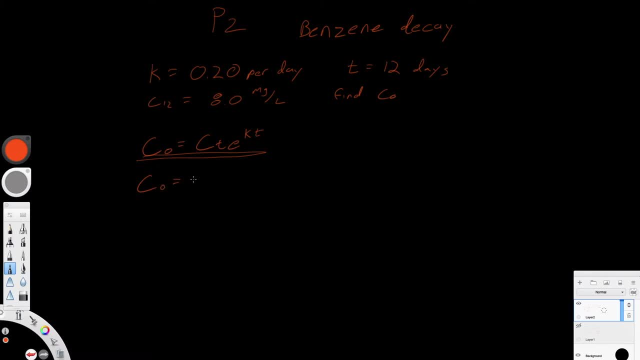 point. this is basically the thing you need to know. so we want to solve the original concentration. so if I get 8 milligrams per liter, yeah E, we have 0.20 per day. I'd just say day times 12 days, and so this is going to be. 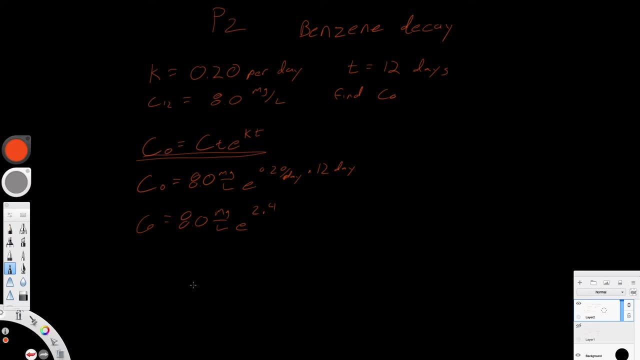 2.4 and then this becomes about. so basically our CNOT is going to be about 88 milligrams per liter in this case. okay, and you know you're going to get probably some kind of combination of this type of question. it might not be trying to find the original concentration, but it's. 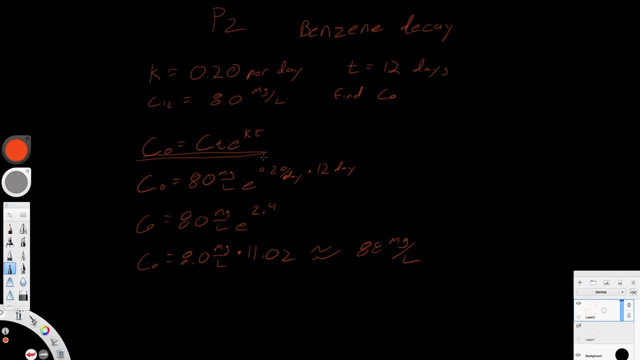 going to be one of these variables that we have up here, or it's going to ask you, or maybe, in addition to that, ask you about like: is this first order in zero order type of question. all right, our third question. this is going to be about setting up equilibrium coefficients and when you 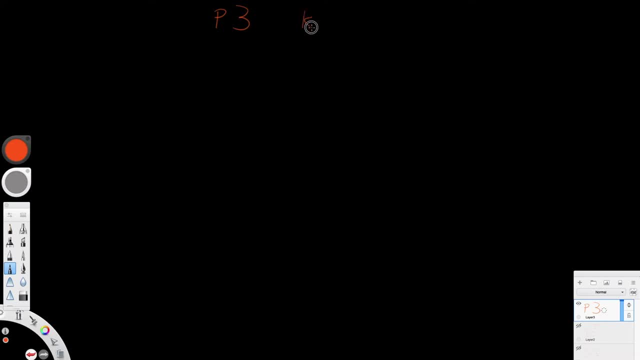 have products and reactants. so in this case, our basic form for equilibrium coefficients are going to be- you can probably hear my kid talking in the background, all right, so this form basically equates to a A plus B, E, C, C plus D, E, and so if we wanted- 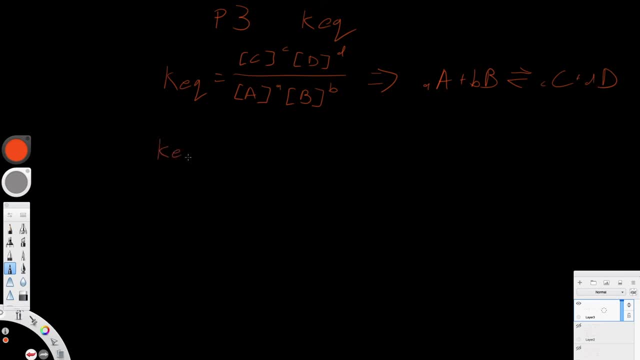 to ask like: all right, what? what is the equation for something like you know what? so is it like like you know? it almost doesn't matter what you ask now, once you know how to do it right, But say something like this: where we have these exponents, 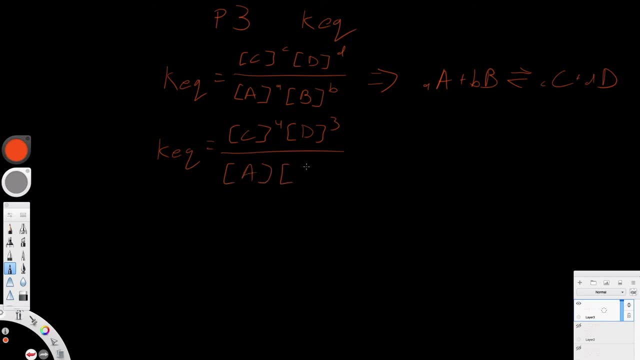 right and now the important thing that you, that is important to remember, is that this is products over reactants. yeah, hopefully I spelled that right. So right, this is going to be the products, this is going to be the reactants, and so, in that case,